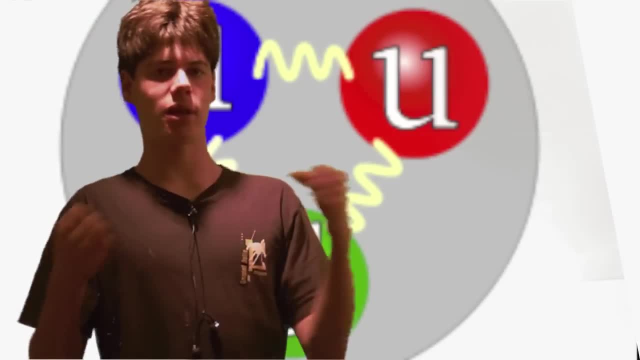 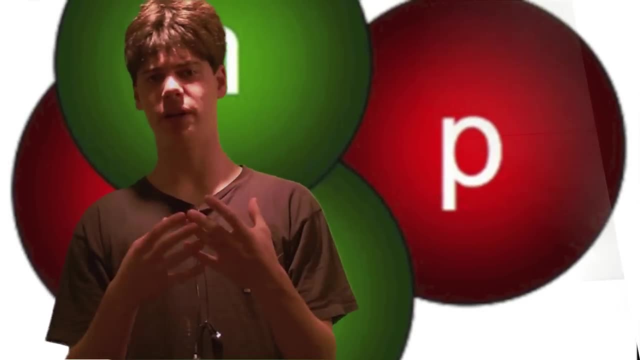 together the quarks in a proton and a neutron. It couples protons and neutrons together inside atoms. It's the strongest force, as its name implies, but it's actually only carried at such a small distance because it's so strong. You can watch the Heisenberg Uncertainty Principle. 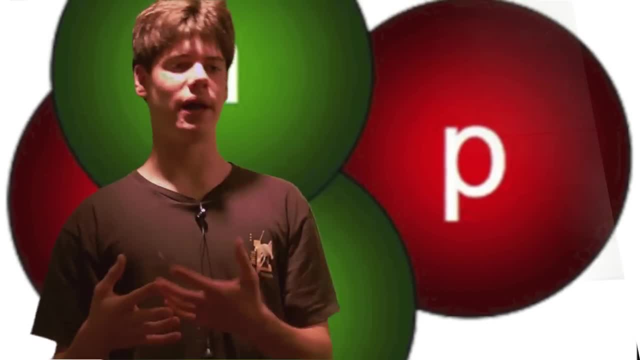 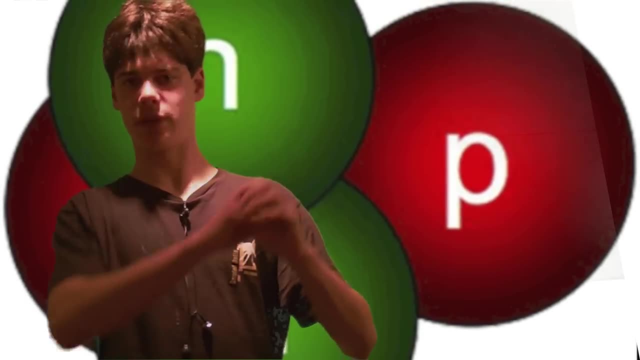 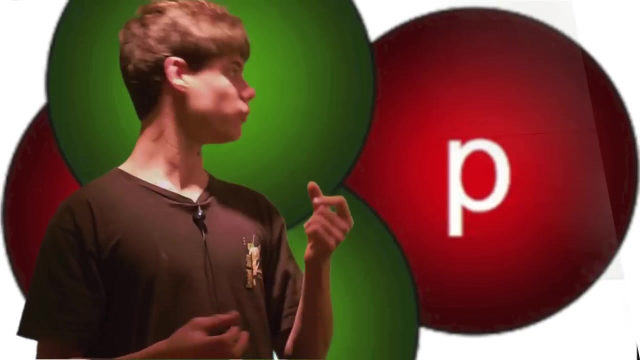 if you want to understand more about why it's only carried at such a short distance. But essentially it's really strong. That's why you never see quarks individually floating around is because that it's so strong that the quarks instantly get pulled together into. 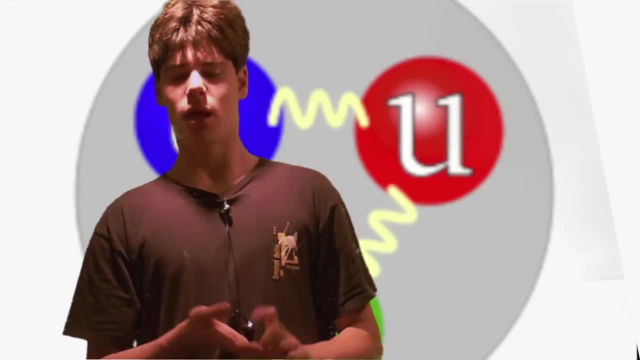 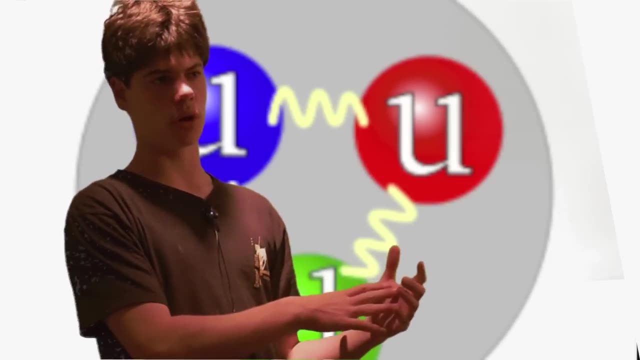 the atom. So it's a really strong force. It's a really strong force. It's a really strong force to a hadronic thing like a meson or a baryon. So what is color charge? How does color charge relate to the strong force? Well, color charge is sort of to the strong force. 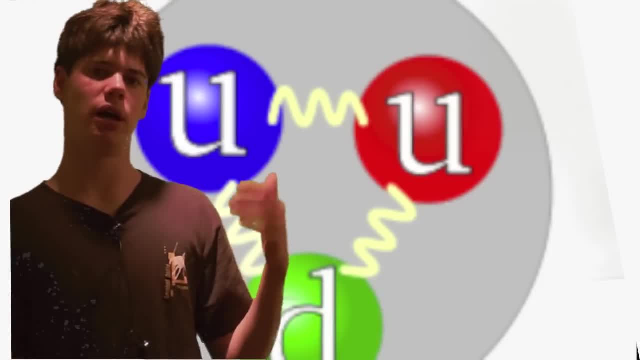 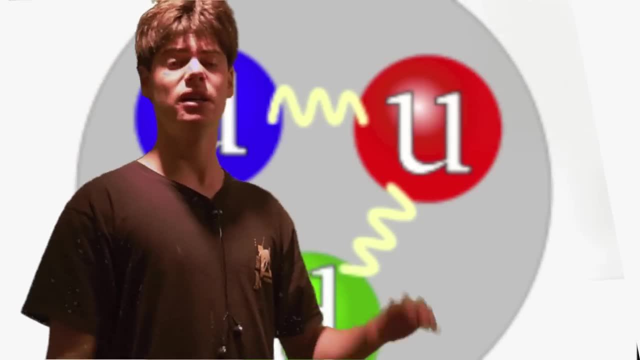 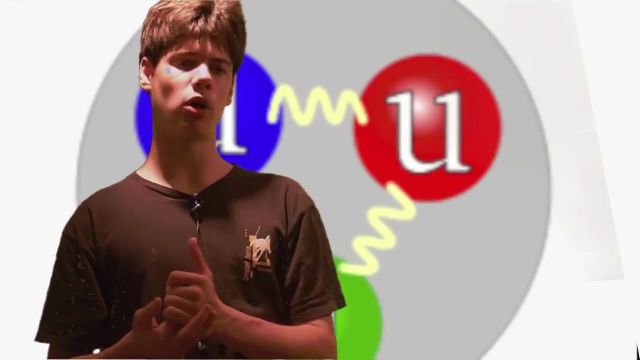 as electric charge is to the electromagnetic force. I'm getting a little tongue-tied, So let's make the analogy okay. It's important to realize that one the word color is chosen somewhat arbitrarily, As really this is not the actual color of the particle, as in like a red quark isn't. 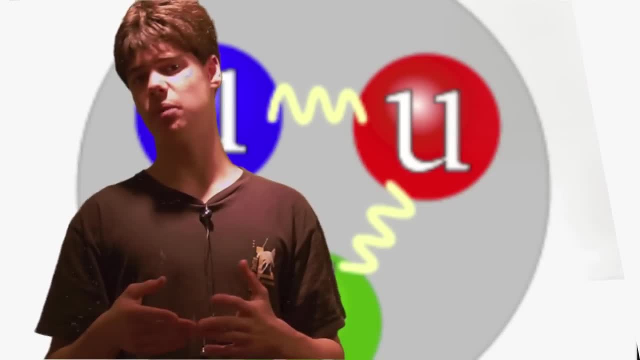 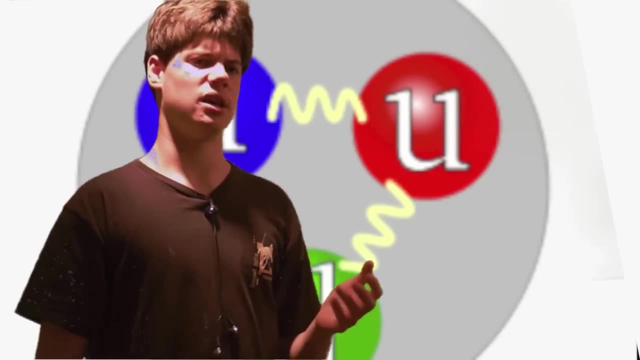 actually red, It's just a name. we've given the color charge and we've given the different states of the color charges different colors, because there's three different colors, like there's three different primary colors. But it's important to note that it's not actually. 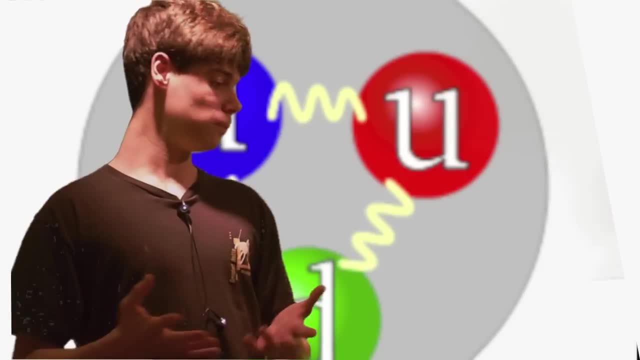 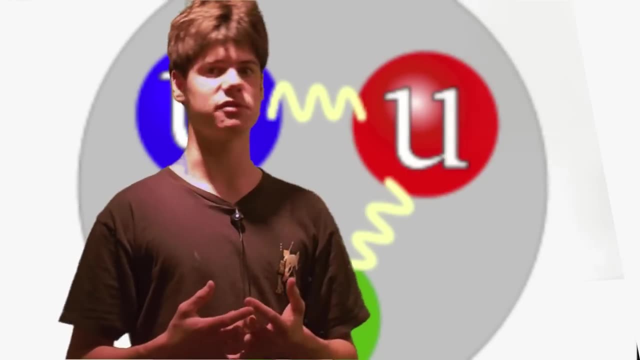 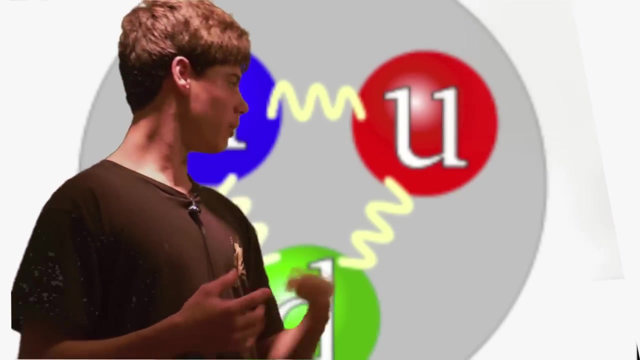 the real color of the particle. So how does color charge create the strong force? Well, it was originally hypothesized because of something called the Pauli Exclusion Principle, which states that no two firm ions can have the same exact quantum numbers. But if you 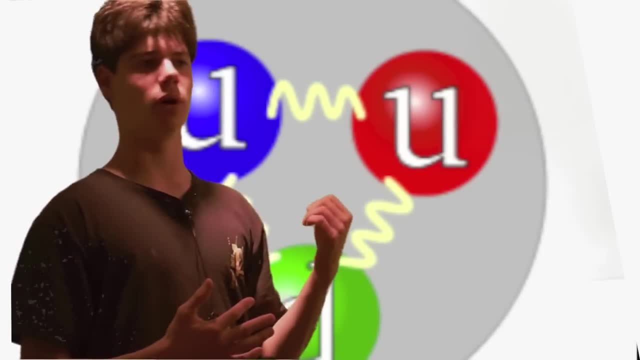 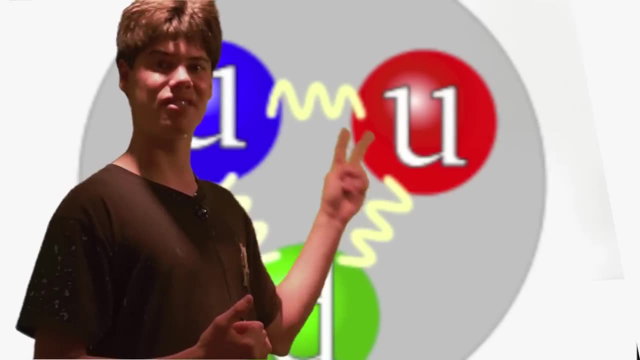 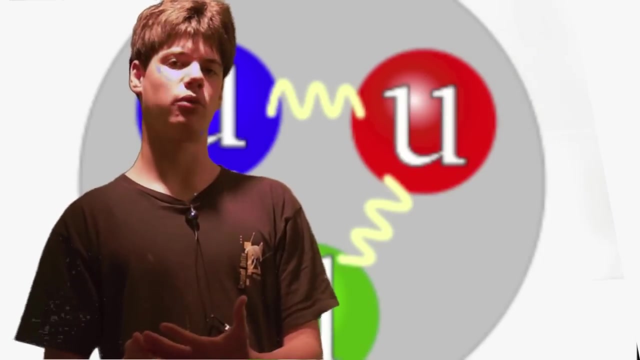 look, there's, say, an up quark, two up and a. what? Sorry, not an up quark, a proton, Two up and one down. okay, So these two up quarks would have the same quantum numbers exactly in this quark. So they thought: well, they can't have the same exact quantum numbers. 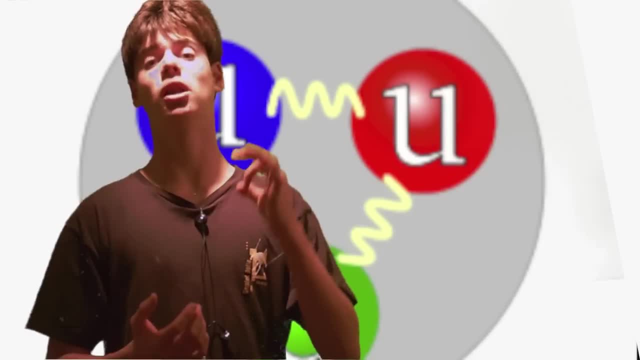 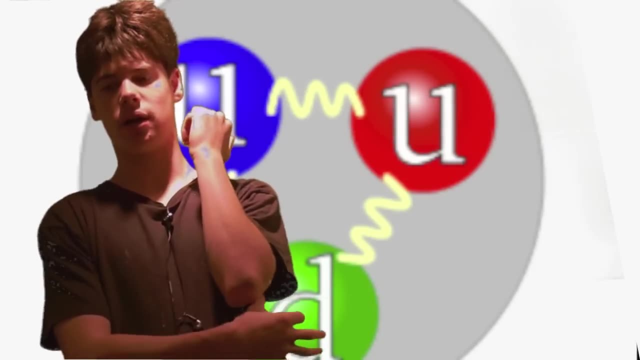 something has to be different. Question from audience, Question from audience, It turns out what's different is the color. So what color does is essentially the difference in color. if you will sort of different colors attract, if you will- I'll explain this in more detail in a second- just like different. 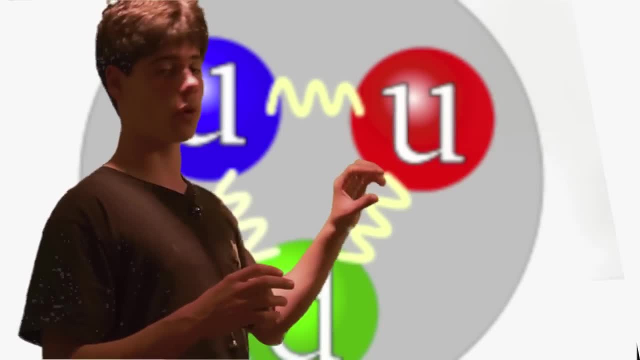 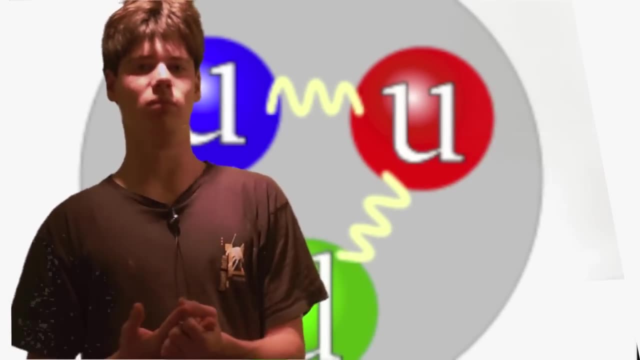 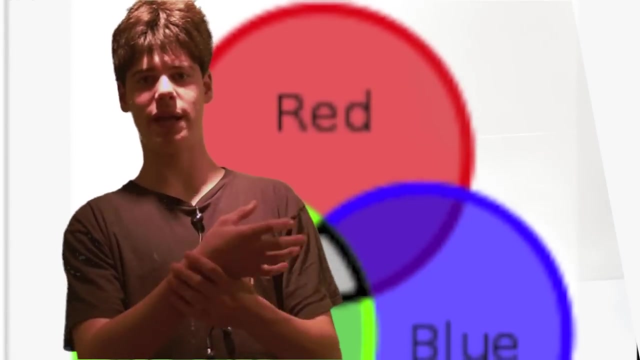 electric charges attract. So these different colors of quarks sort of attract to each other and this strong force pulls them in. So that's the analogy. it's sort of like the three different colors are like the electric charges. it's the electric charge creates the electromagnetic force due to attractions. 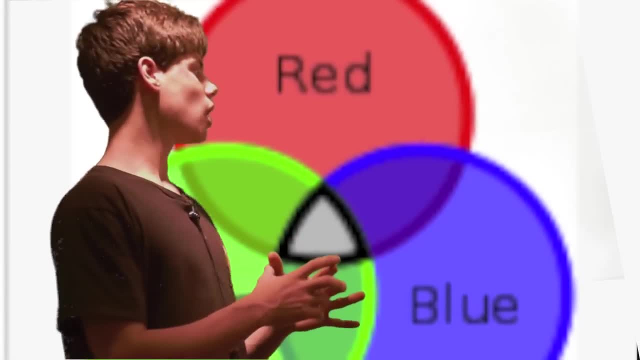 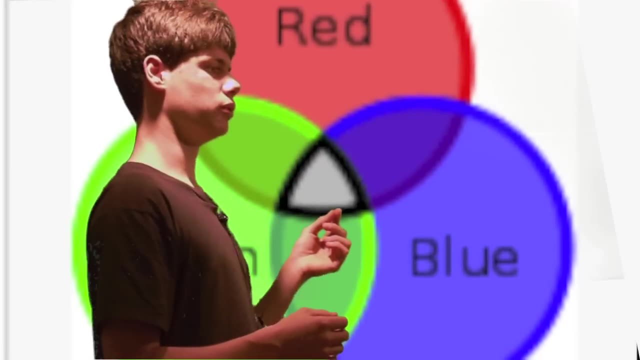 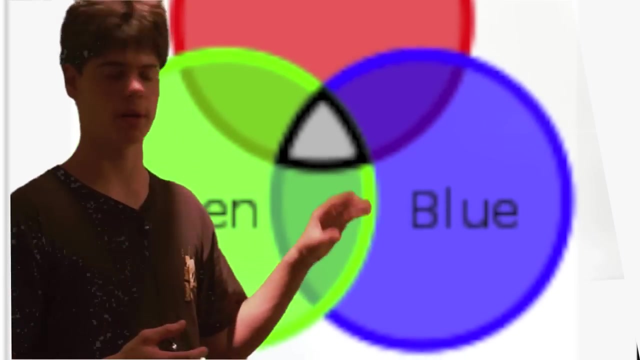 between charges. So what really happens? Well, color charge. a quark can be either red, green, red, yellow or blue, I believe. So red, yellow or blue could be actually red, green or blue. sorry, RGB red green. 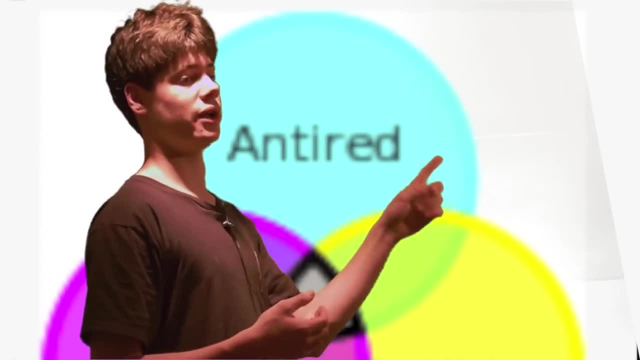 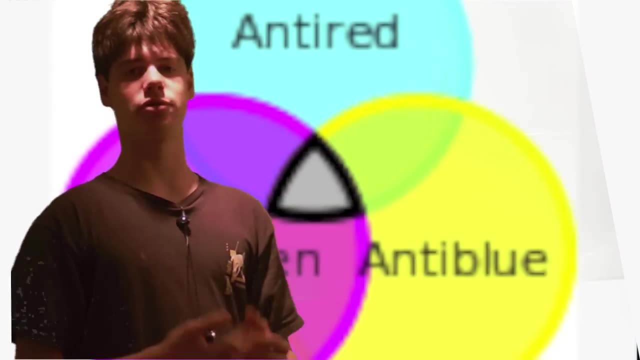 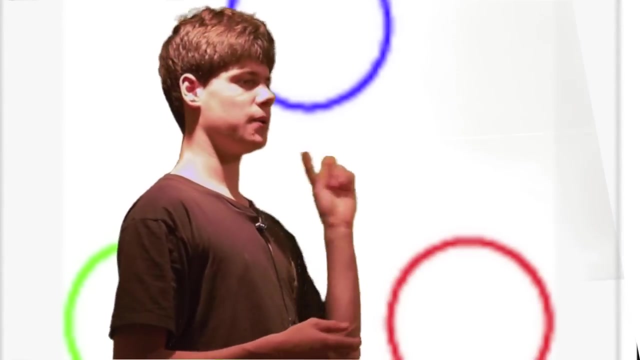 blue, three primary colors, And it can also be anti-red, anti-green and anti-blue, which are like the whatever reverse colors if you will those colors are. So say, we have just any baryon with a red, green and a blue quark, okay. 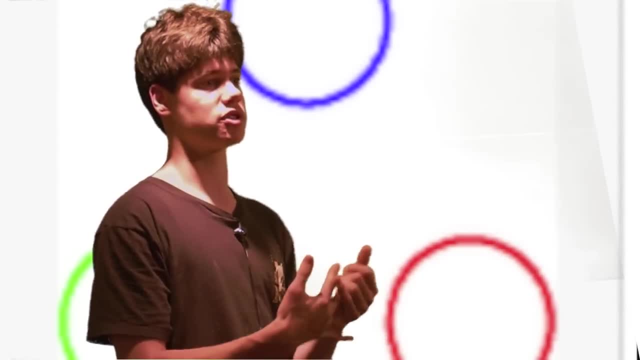 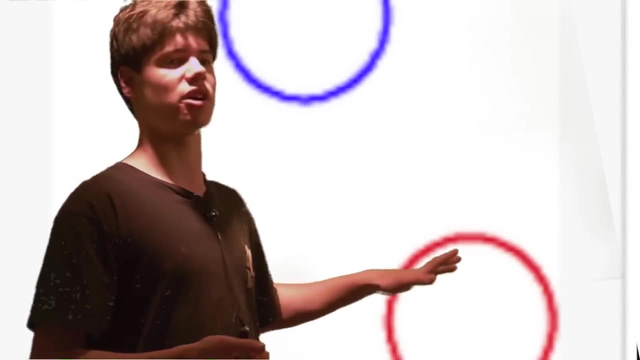 You also know that gluons transmit the strong force, So gluons can have a combination of two, so like red and anti-green. okay, Gluon is a red, anti-green gluon. okay, a combination of both the red and the anti-green. 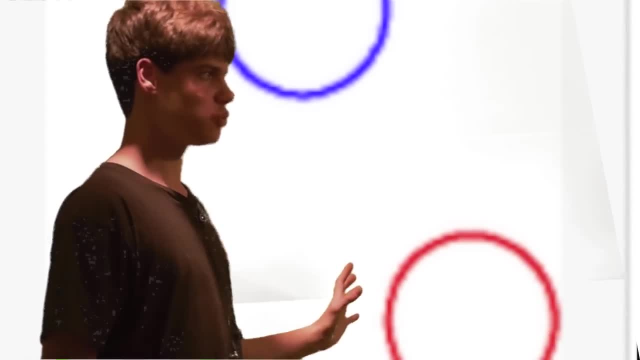 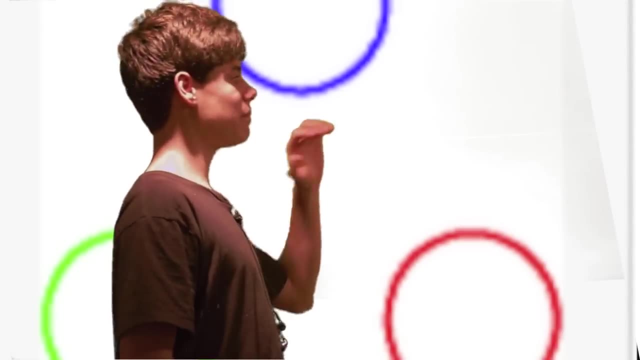 okay, What happens to cause the gluons to switch? Well, we have a red, green and a blue, okay. So what's going to happen is say we'll just focus on the red and the green for now. okay. 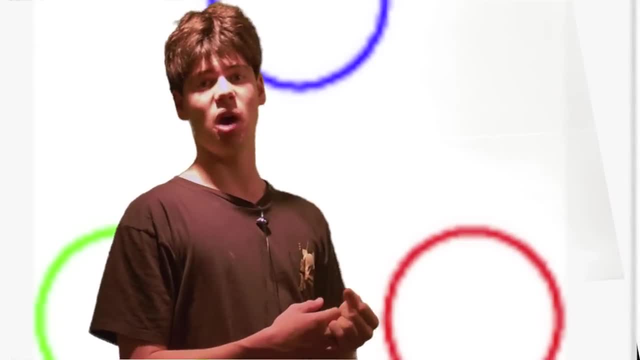 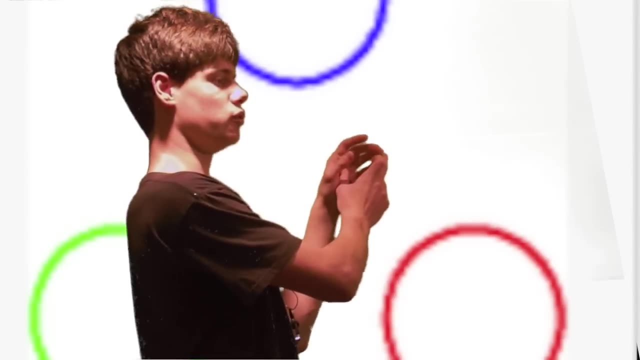 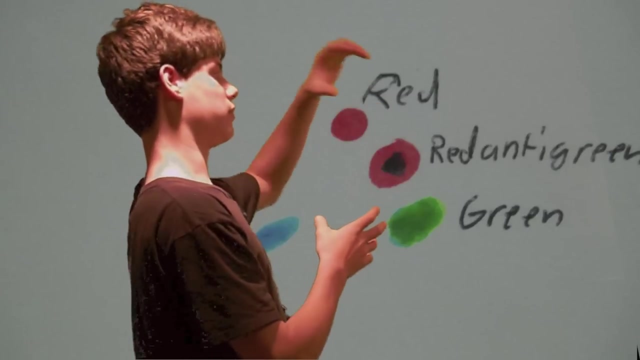 So say the green. okay. these are taken from Wikipedia, by the way, these images, So say the green quark. what it's going to do is it's going to emit a gluon, okay. So what's going to happen is the red quark is going to couple to the green quark, okay. 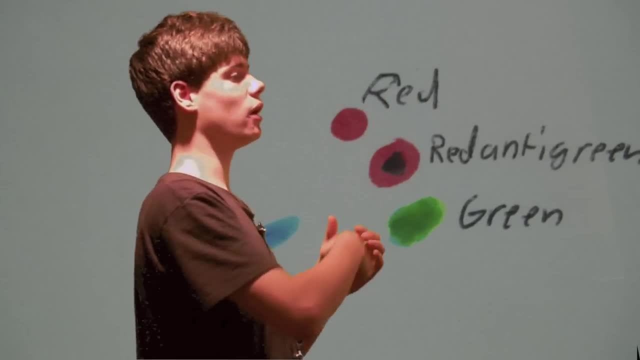 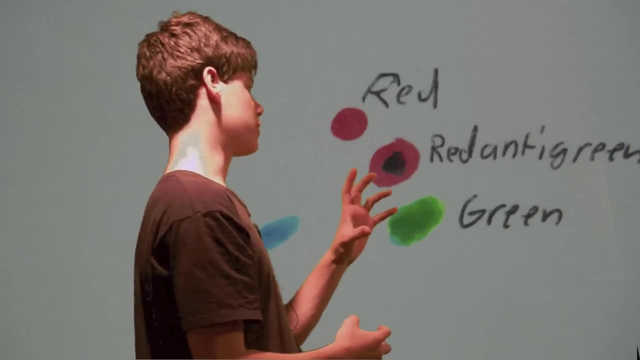 And the way it's going to do this is it's going to emit a gluon that is red, anti-green. okay, So what happens is the gluon is red and anti-green. So what happens is you can think of this red quark as it gets rid of the red color charge. 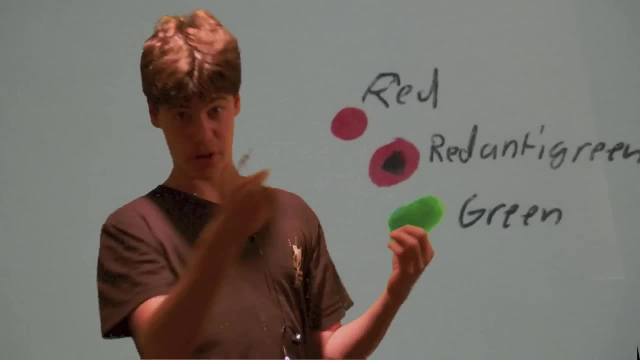 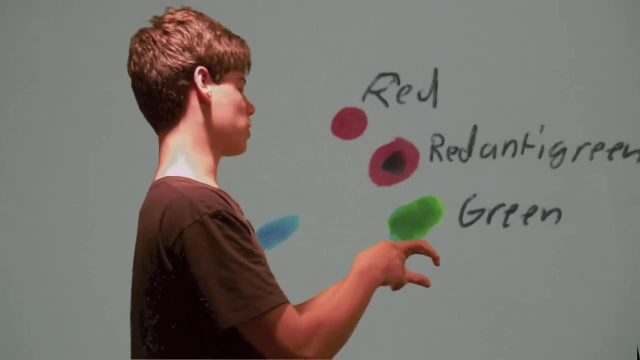 through the red gluon and it gets rid of the anti-green charge and the getting rid of and the anti sort of cancel each other out. Okay, So it becomes green. And then this green quark, this green, the green of the quark and the anti-green of the. 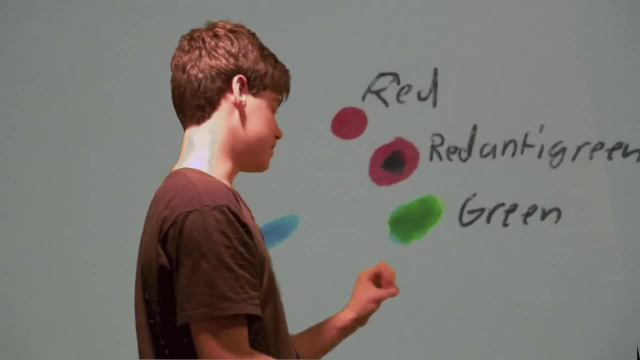 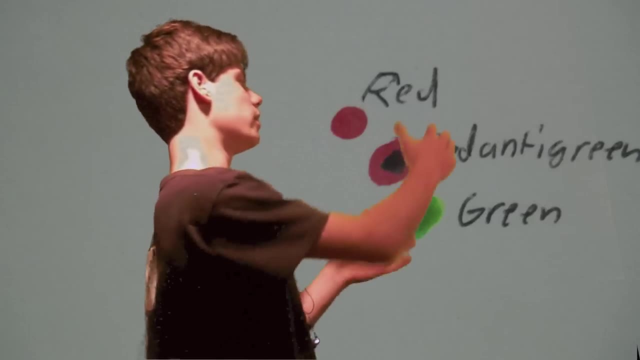 gluon cancel out, and then the red of the gluon is then the new color of this new quark. It's not the new quark, it's the same quark, but it has a new color. So in other words, they flip-flop color. 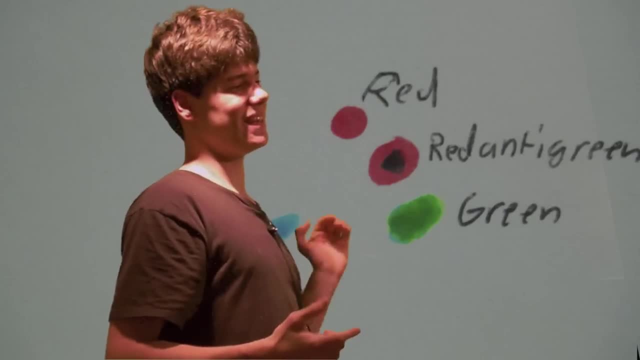 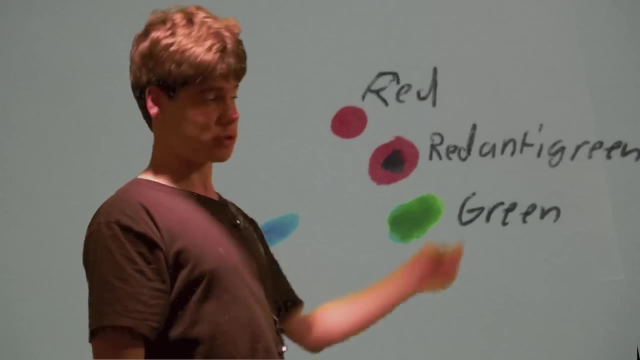 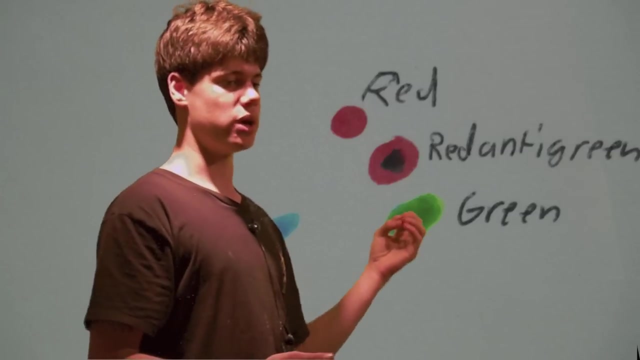 And then this is what keeps them attracted to each other, because they keep exchanging gluons to keep color changing is what it's called. It's called: keep flip-flopping the colors between all three of them, and that's what creates the strong forces, essentially the attraction between the different colors. 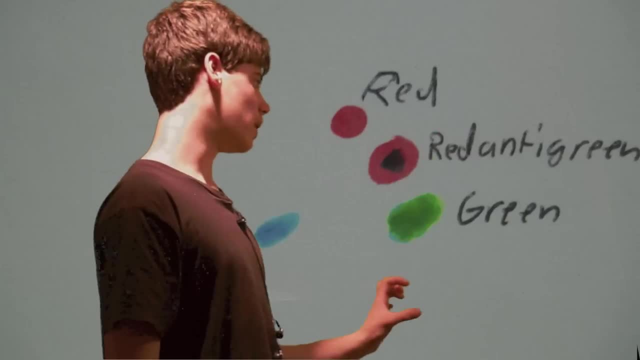 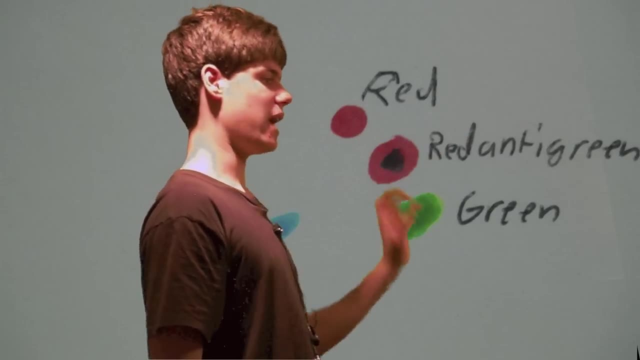 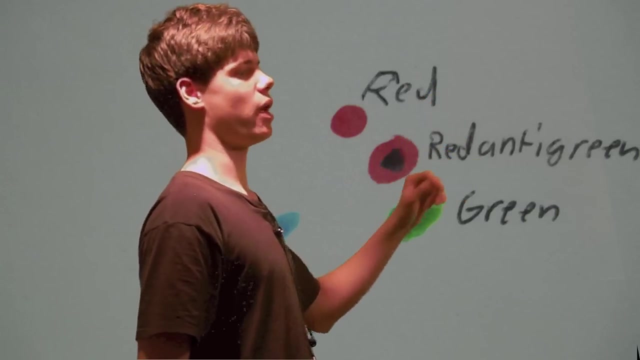 Okay, That's how it works. is you have these, the gluons and the quarks, sort of flip-flop colors? by emitting their color and emitting the anti-color of the one that it's going to? So if you had red and blue, the blue one would emit a blue anti-red. 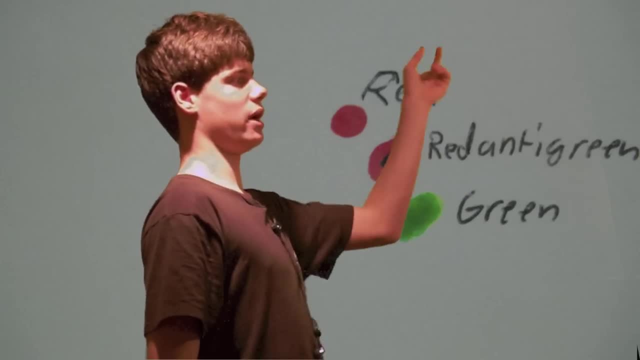 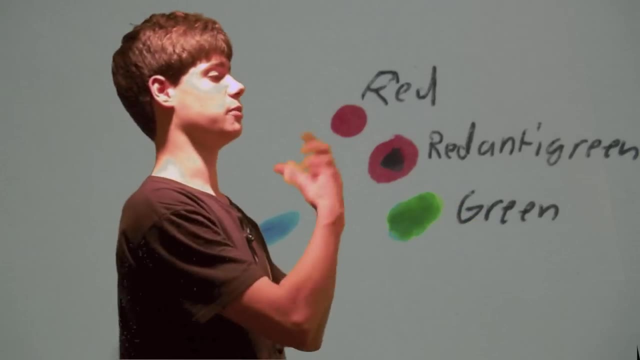 And then so it would get rid of the blue and get rid of the anti-red, which means it would become red itself, And then the red quark, it was going to the red, the anti-red would cancel out and it would become blue. 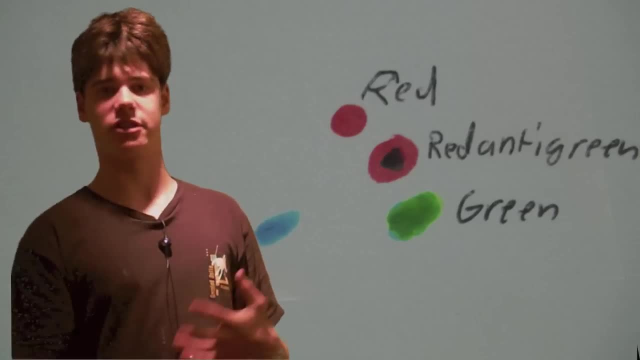 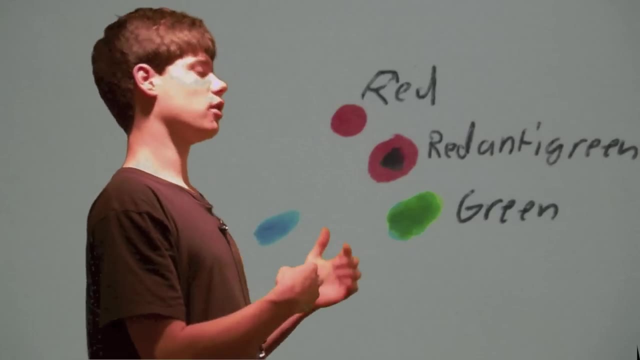 So that's really all color charge is. I'm sure there's complex mathematical things that I don't understand myself, but that's really all it is. So just to sum up real quick here: strong force is what couples things together. The strong force itself is caused by the coupling of colors. 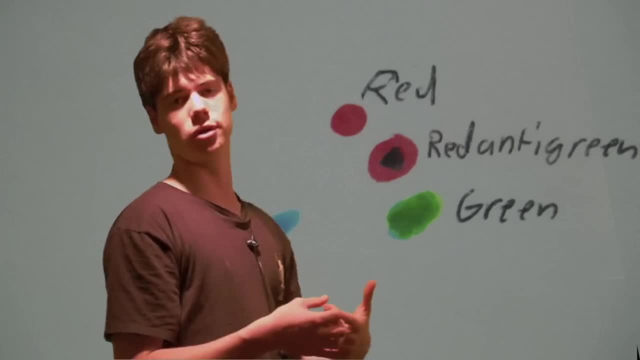 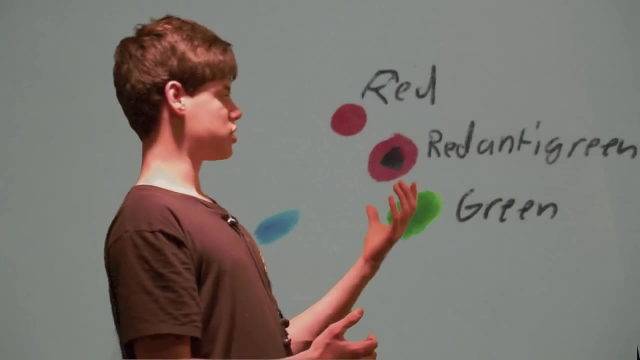 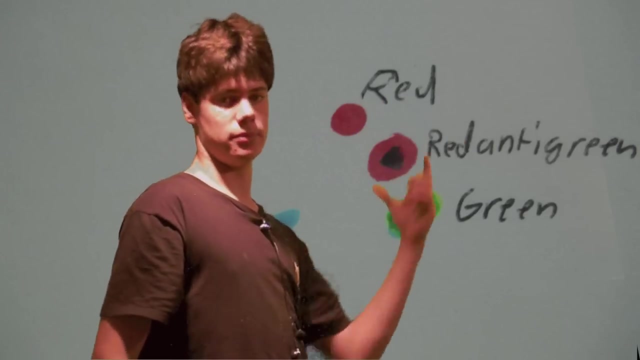 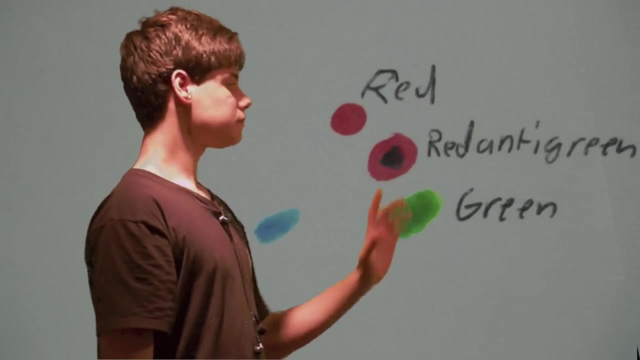 Okay, Okay, Okay, Okay Okay. The attraction of different colors in quarks or anything that works by the strong force. And these different colors are attracted because they are different and differences attract, and they exchange gluons and they keep flip-flopping colors, or color changing, if you will. 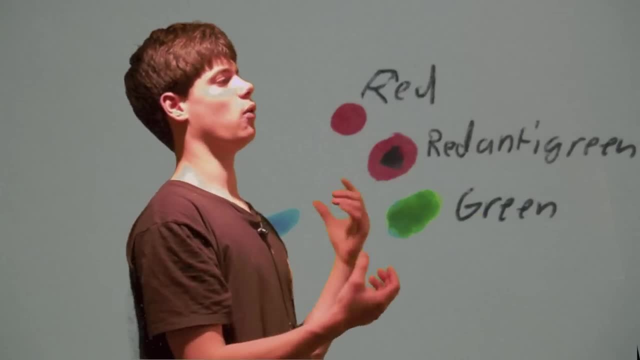 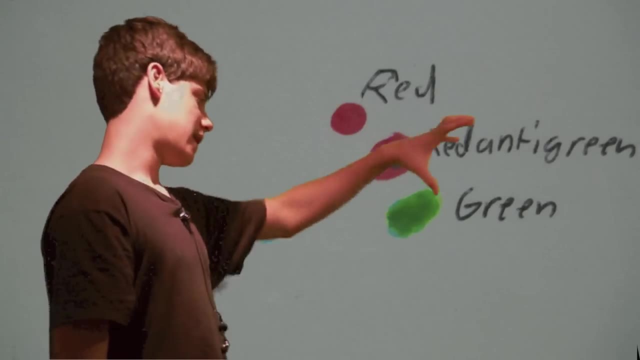 And this creates this. this is what a hadron is or a meson actually is, when a quark is a quark and an anti-quark. It works with mesons as well, but they keep flip-flopping colors And but the important thing to know is that one assumes the color of the other one and